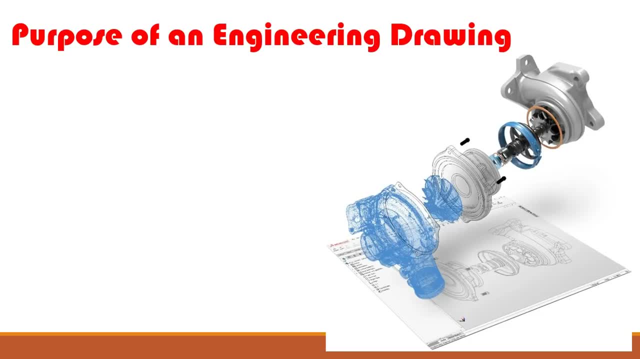 You know, they usually think of it in terms of what their responsibilities are, whether it's to actually manufacture the component, whether it's to inspect the component, whether it's actually to quote on the component. but it has a whole variety of uses. that makes it one of the most valuable tools in the manufacturing and design process. 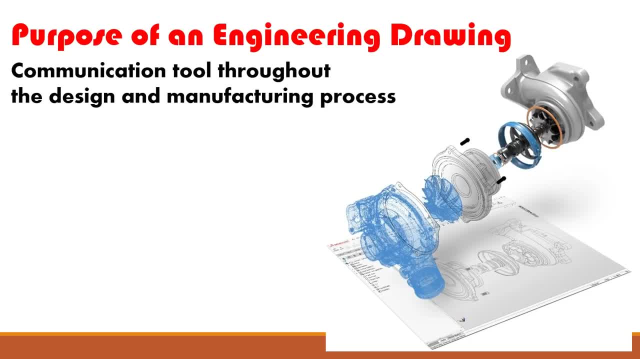 So it's a communication tool, you know, throughout the design and the manufacturing process. It's specifically and literally a method that you can communicate the life cycle of a product without two people actually interfacing. It has as much information on it as a well-written letter or as a video or as two people actually talking, and a well-done blueprint can communicate everything about a part and it's, you know, essential to anyone in the manufacturing process. 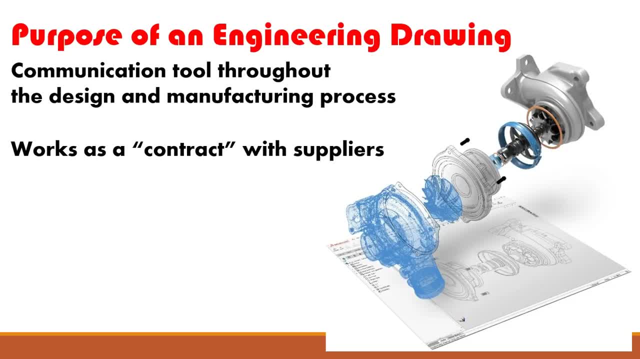 It works as a contract with your suppliers. I had several examples when I was working in industry where I had a part that came in and it wasn't done to specification and, instead of getting into an argument over why the part didn't look the way I wanted it to look, 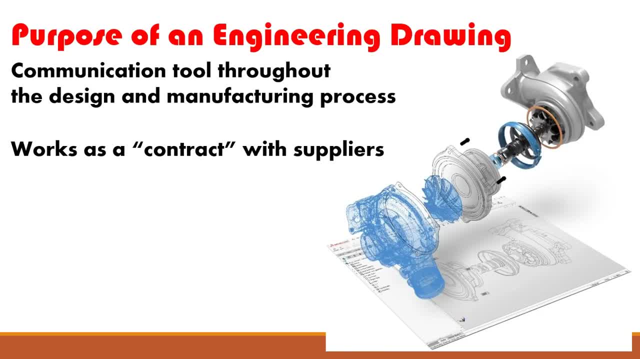 I could just call up the blueprint and point to the. you know the features that were in question and there was no longer an issue with the supplier. You know it worked just as well as a contract. It said what my intentions were. 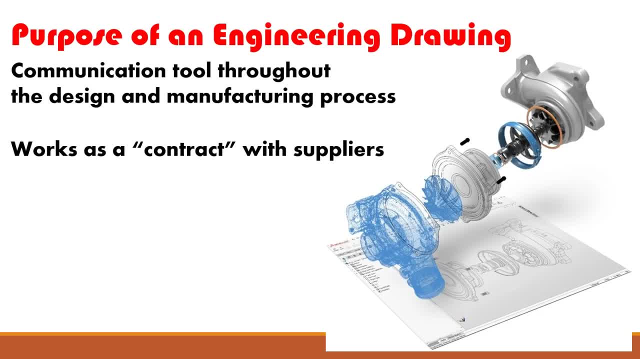 It said what I expected, what the deliverables were. It actually, You know, communicated a lot of information that was indisputable because it was a well-done blueprint. It establishes the acceptable part: quality. Now, you know, a blueprint obviously is going to have a lot of dimensions, a lot of, you know, different types of features in terms of the type of quality, the type of surface finish. 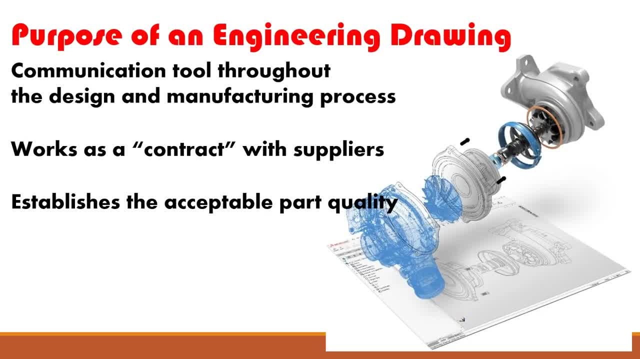 So it gives you all the things that you would need when you consider this a good quality or a poor quality part as a customer. So the customer determines the quality And that is how you determine what you're going to get as a good part through that blueprint. 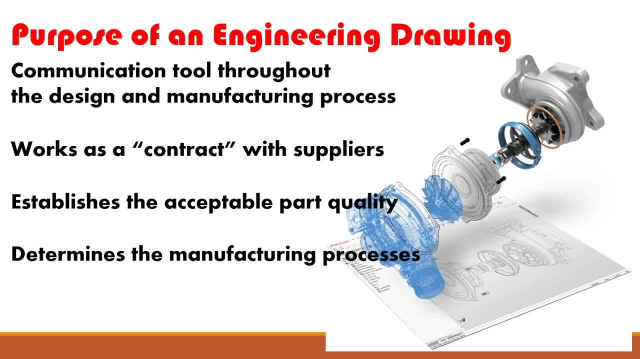 It helps determine the manufacturing process. Now you think, well, how does this dictate the manufacturing process? Well, a lot of the thing- issues with tolerances that you see on a blueprint- can only be achieved through certain processes. So if you've got a certain tolerance going out to a certain number, of certain amount of precision, you know the number of decimal places that are on your tolerances that dictates whether or not you can machine the part. 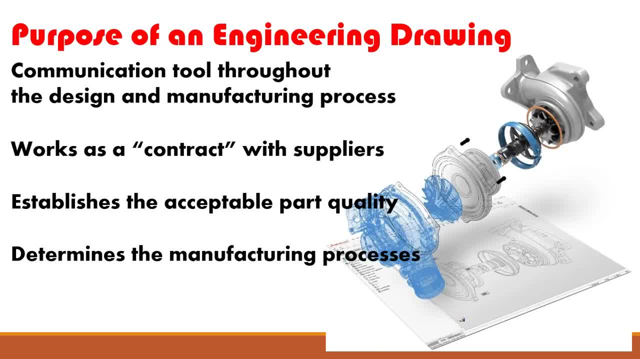 Whether or not the part has to be ground, whether or not it has to be polished or whether or not it's going to be acceptable as a cast surface. So you know, based on the types of tolerances, the types of surface finishes that you call out, you know it really does narrow down and help you determine which manufacturing process is going to be acceptable. 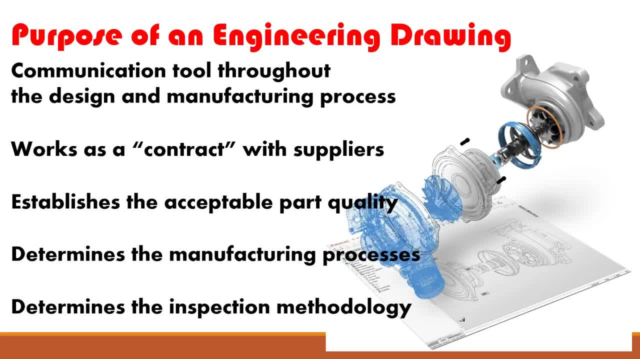 And last, it determines the inspection methodology. So again, it goes back to how you're going to clamp the part down using your GD&T, And if you want to see more of that, you can go to the GD&T website. And if you want to see more about geometric dimension and tolerancing, I have a couple of videos that you can watch and a whole playlist of GD&T rules and fundamentals. 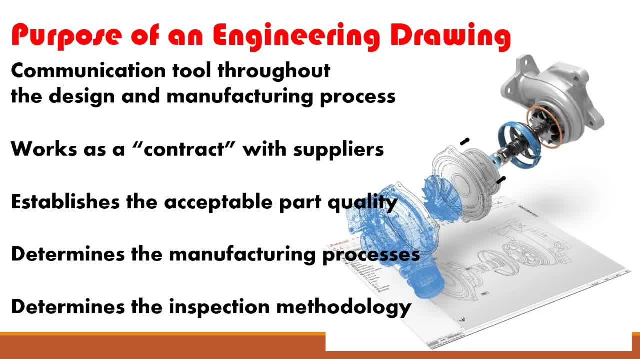 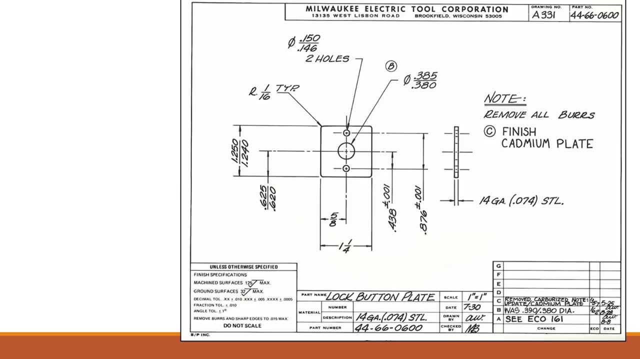 But it also lets you know. you know how you're going to clamp the part you know, and what features have to be held in relation to which, as well as the entire inspection process, can be dictated through the blueprint. Now, what we have here is a very simple blueprint. 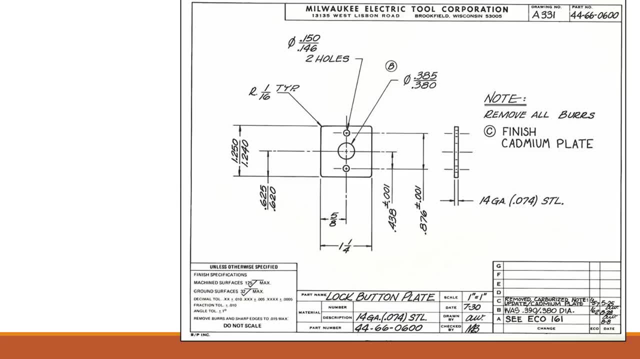 It's for a product called a lock button plate. You can see it's one quarter of an inch by one quarter of an inch. You know there's, you know, some little idiosyncrasies in this drawing, but I think it serves its purpose. 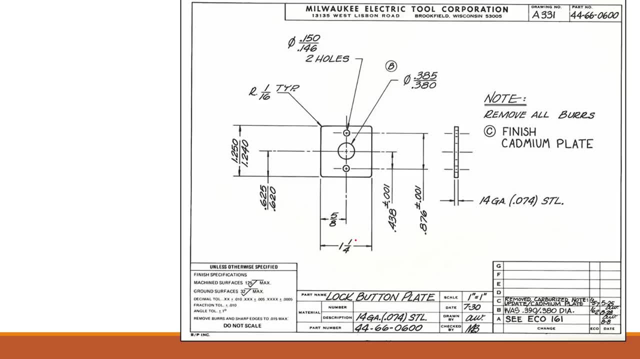 What I really wanted you to see is all the essential components of this blueprint and why it's actually a very good blueprint. It has three components that make up a good blueprint. that actually gives it all the information for manufacturability. It gives it all the information for inspection, as well as makes it a solid contract if you were to outsource this. 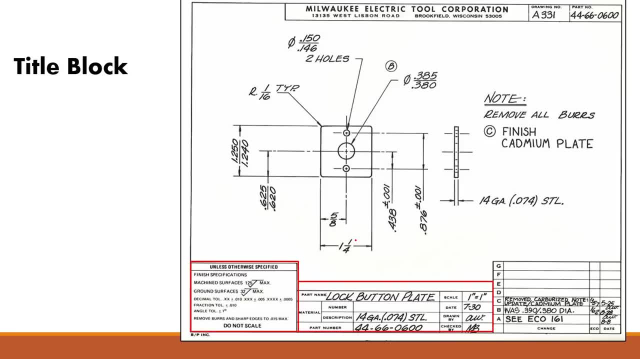 Now let's look through some of the what those three components are. First, it gives you a title block. A title block is the information that lets you know about the company as well as the drawing You know. when you look at a title block, you'll know who. you know not only what the part name is, you'll know any part numbers, who the engineer is. you know the scale that you're looking at the part at. 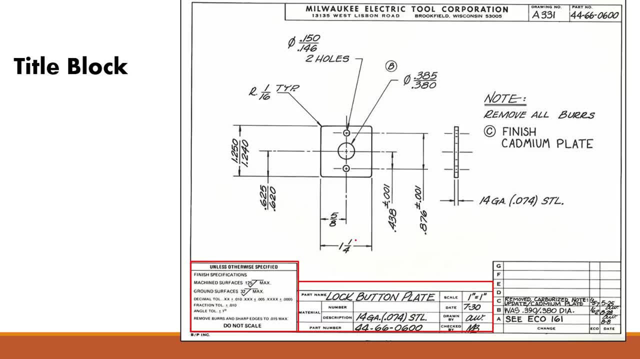 and any crew. You'll know what the part name is. You'll know what the part number is. You'll know the initial tolerances for that part. There's also a revision block. This is extremely important in terms of contractual disputes. You know what it tells you is what changes were made, when they were made, a date that they were made, as well as who approved those changes. 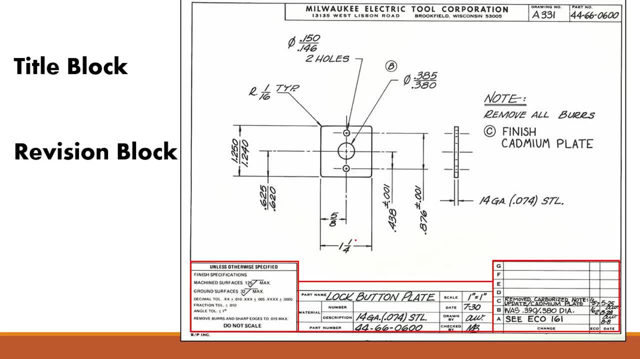 So if you have a part that comes in that's not made to your current specification, you can cross-reference between when that part was ordered and when those changes were made in the revision block, So that way you know it can protect you as well. 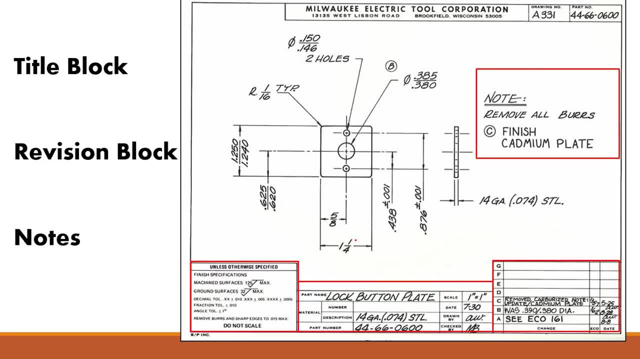 As well as the supplier of the component. And then any notes- Now, notes is a very generic term. What that is is just any extra information that doesn't quite fit in the title block, doesn't quite fit in the revision block. 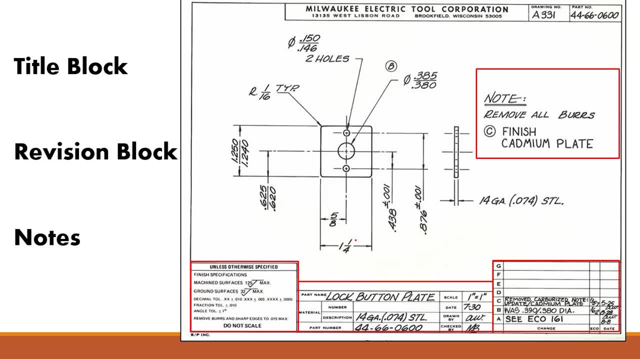 You know things such as removing all bears. You know unless specified. You know all these sorts of information that you might need that you want done to your part that isn't going to readily be available in the title block Or any part that doesn't fit in the revision block. 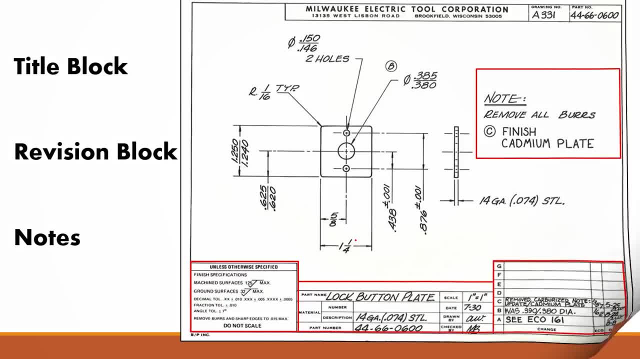 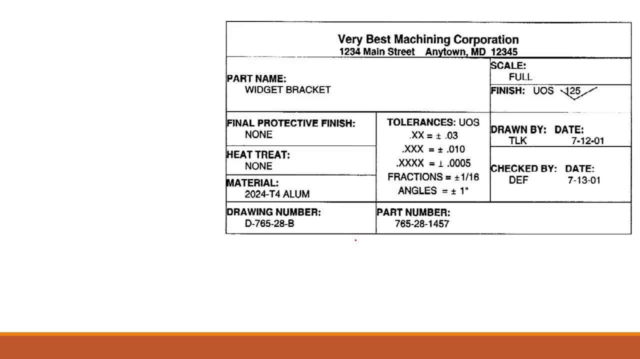 Or any place else on your engineering drawing. So let's look at a title block. So the title block- you know, one of the more crucial parts of a drawing- has several components that I want you to become familiar with. So you got this title block. 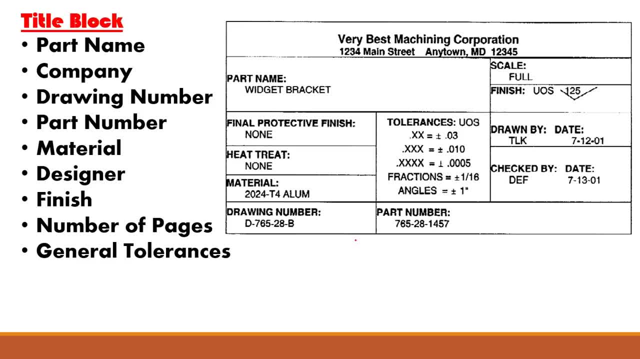 Several things you can find. One is a part name. So let's see if I got my widget here. So you got a part name that is part of the title block. So this way everyone knows exactly what they're talking about. 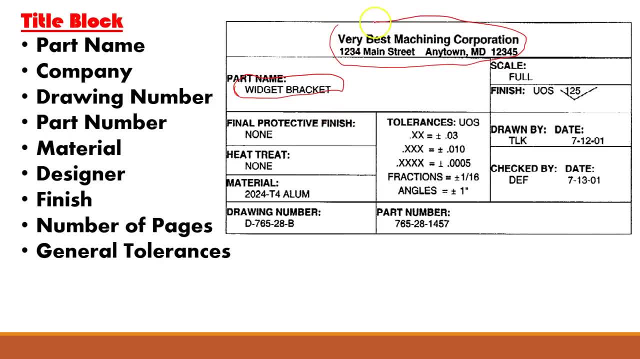 The company name is typically in the title block. It can be somewhere else in the drawing, but it usually it's in the title block, A drawing number and a part number. This is very important. You'll see this particularly in large companies that have a lot of components that they're concerned with. 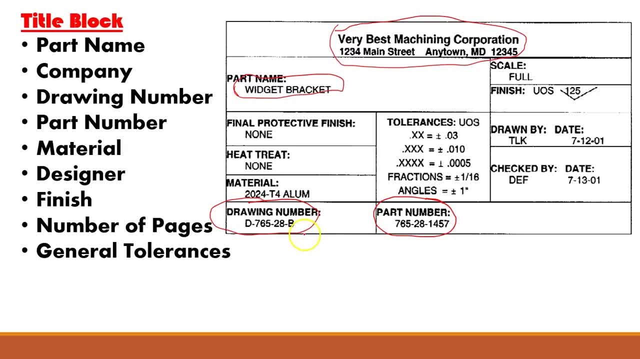 This lets you know. you know not only which drawing you're dealing with and which page of the drawing, but also if you've got different families, So you can say: okay, which part number am I speaking of? precisely The difference in part number can be the difference between the two. 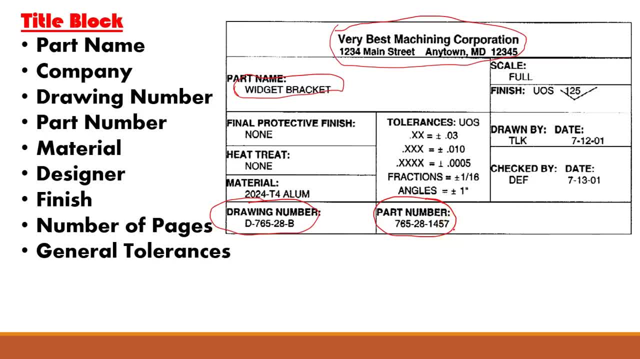 It can be the difference between two parts that look otherwise the same, but they might have one or two very crucial features of difference. You also have the material Here. we can see this was made out of 2024 T4 aluminum. You have the designer, as well as the person who checked it and the date that they both did that. 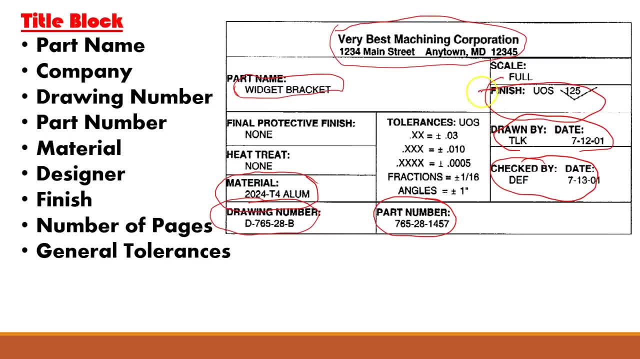 You have any kind of finishes. So here we've got a 125 surface finish. We also have whether it's going to have a protective coating. So here we've got a 125 surface finish. We also have whether it's going to have a protective coating. 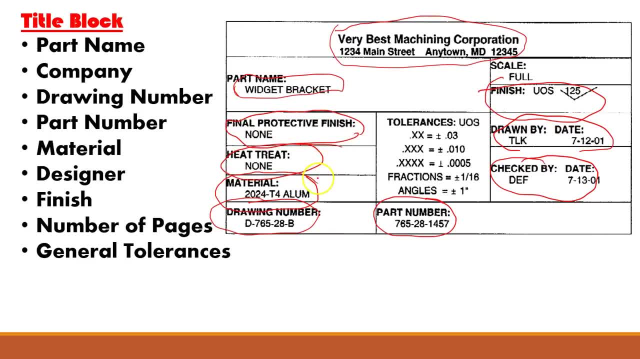 We also have, whether it's going to have a protective coating Or heat treating. You got the page number, So if this is a drawing that's going to be part of a series of pages, that'll show up in the title block. 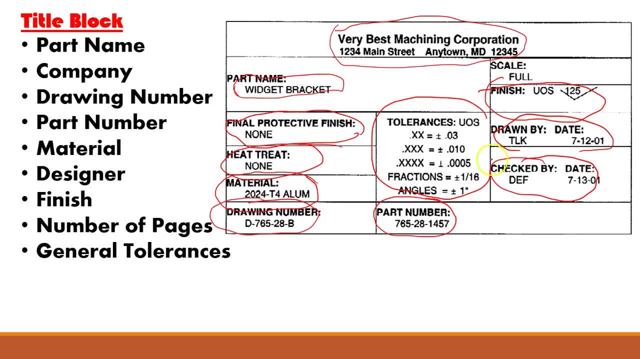 And you have what is here is general tolerances. So, as you can see, in most drawings they'll have a tolerance and specifications on the actual component. But if you have a drawing, a more universal tolerance that you want just carried on throughout, you can cover that in your title block. 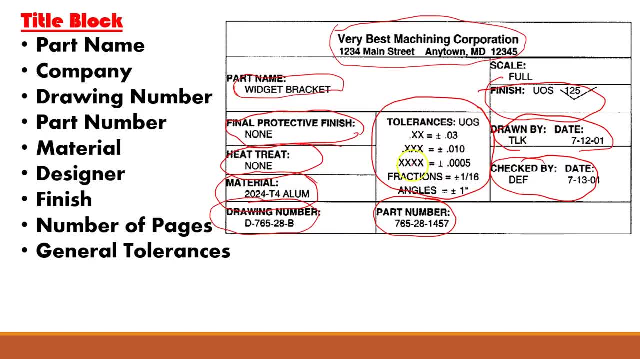 your title block. so here you've got the tolerances with the precisions, which helps you dictate what kind of manufacturing process and any type of angles and other types of tolerances that might be universal to the part. so this is a very crucial portion of a drawing. 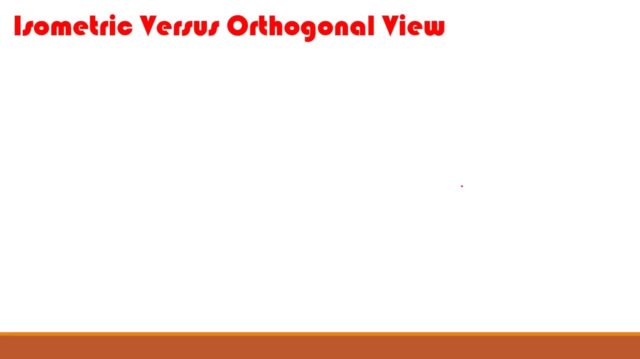 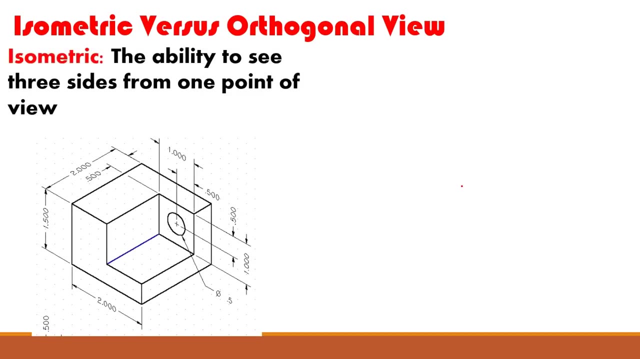 now, one of the more important parts of drawing is the isometric view versus an orthogonal view, and it's also one of the simplest to understand. so an isometric view, it just gives you the ability to see apart from three sides. you know, it's that ability to look at a drawing and say, okay, i can. 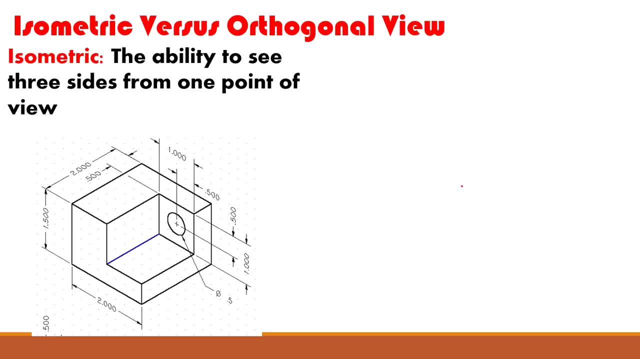 look at this particular drawing here and know whether or not i'm you know what features apply to the top, front and side. so you've got a top, front and side. you also have some dimensions on it. you don't necessarily have to have dimensions on on any of these views on the. 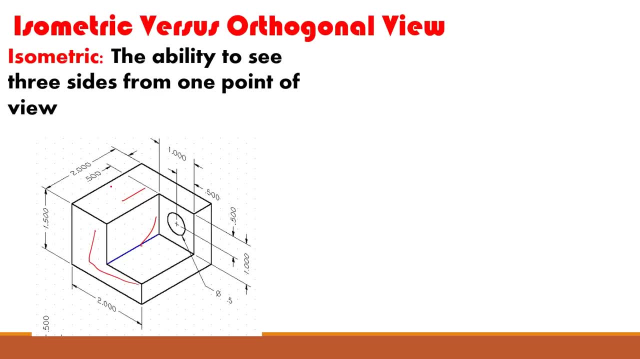 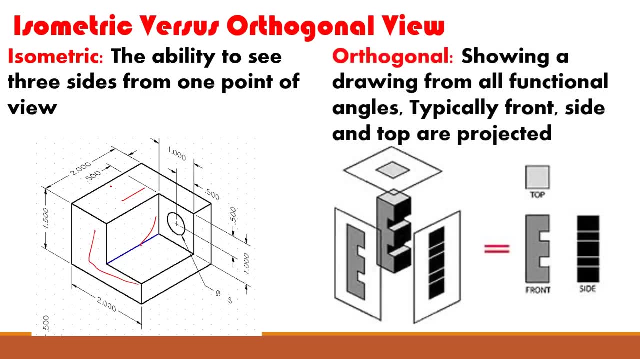 isometric view in particular, but this helps give you a good visual for how this, how the component is made and how the sides are- relate to one another. now you've got an orthogonal view and it shows the drawing you know as a function from different angles, so different types of 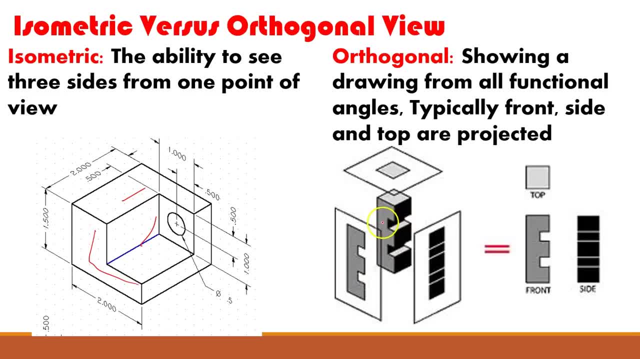 projections. so here you have this big three-dimensional letter e and in an orthogonal view you'd have a very specific front that you're looking at, just looking at the front of the e. you have a top that you're looking at, looking at the top of the e, and then you've got 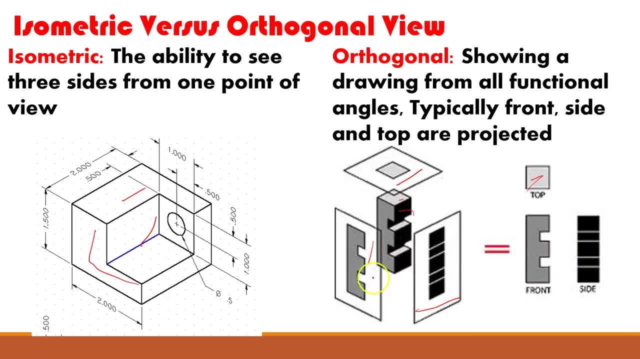 this side view which gives you some ideas, the side of the e, and i think i got these back, so this would be, excuse me, the front side and top. okay, so that is. you know you could picture this being part inside of a glass box and as you look at one side of the glass box to the other, that 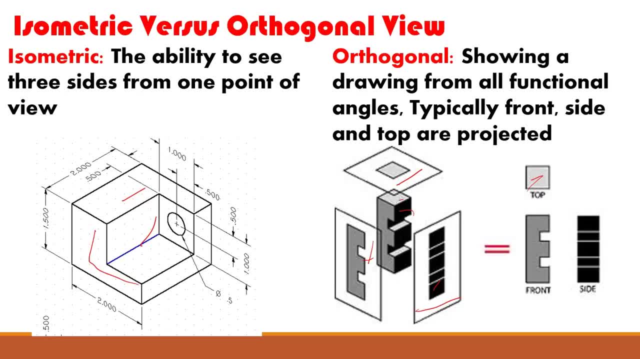 gives you. you know whether or not you've got what portion of the orthogonal view you're you're looking at what you're actually concerned with. so that is the isometric view in the orthogonal view and this will show up in all the other drawings. well, these are like two general categories of. 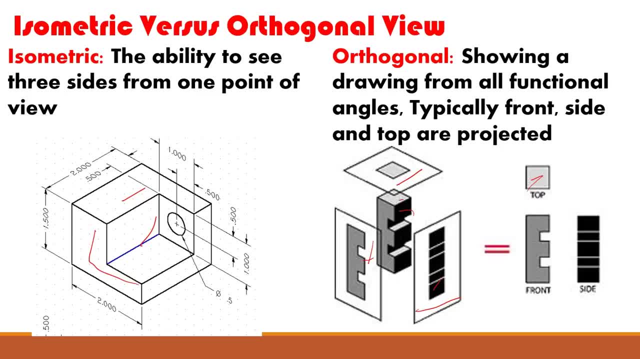 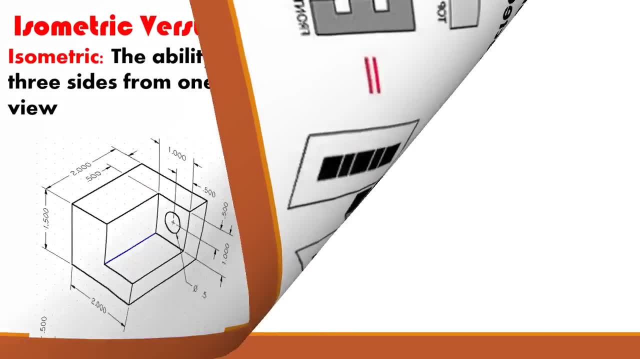 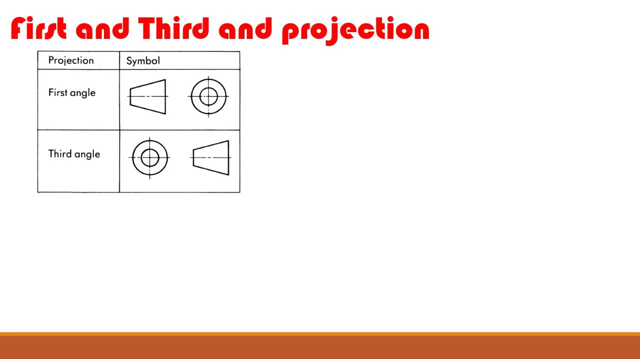 drawings- and you'll see this throughout most engineering drawings. you'll have them based on an isometric or an orthogonal- orthogonal point of view. one important thing that can be very confusing- and it's mostly, i think, confusing, depending on where you learned your engineering drawing from and where you first started seeing engineering. 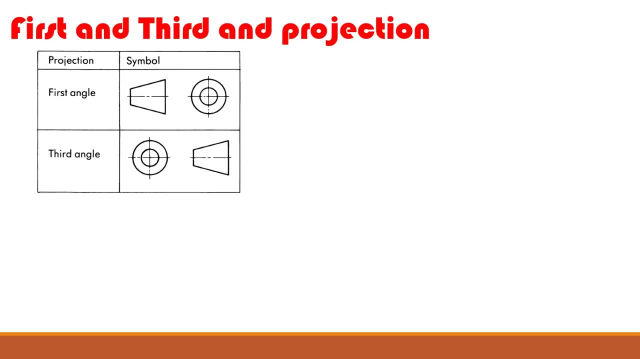 drawings where you've actually worked is first and third projection. now, the first and third angle projection is just a different type of notation: how drawings are set up, particularly for, you know, orthogonal drawings. what you have here is a first angle projection, third angle prediction. one is more common in the us and third angle view is more common in europe. 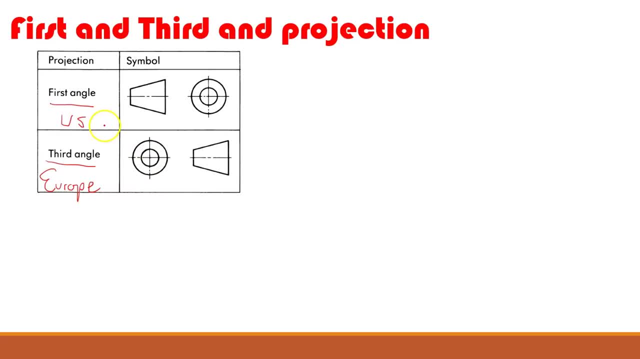 you know, in different parts of asia. so us and i believe, uh, just all of north america, and the third angle view will believe, is a a european and and parts of asia. now, the way you can think of these two projections, if you consider, you know, break the universe up. 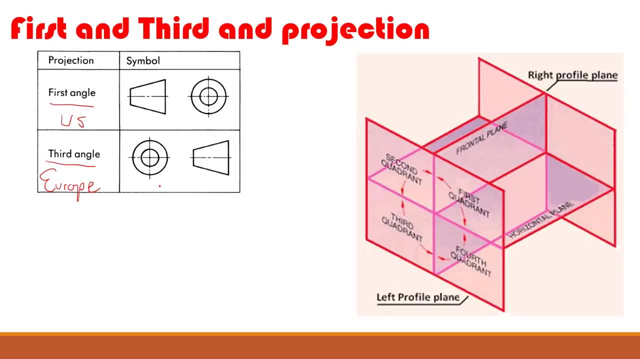 with a left plane profile plane, a right profile plane, a horizontal and a vertical plane and you think everything has to be positioned in a different quadrant of these different planes, you can start to understand your first and third angle projection. so first angle projection takes place in this first quadrant, so right here in the first quadrant, third angle projection you picture. 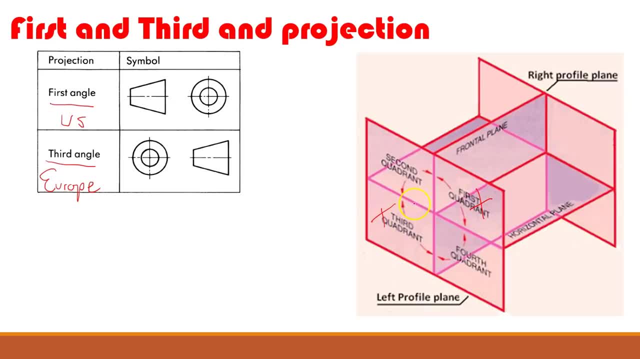 your object in the third quadrant and you, as the observer, are always in the second quadrant. so here you are, standing in the second quadrant, viewing both first and third angle projection, and your object, whatever it is you're looking at, is still in the same orientation. it's just either going to be portrayed in the first quadrant or the second quadrant, so you don't. 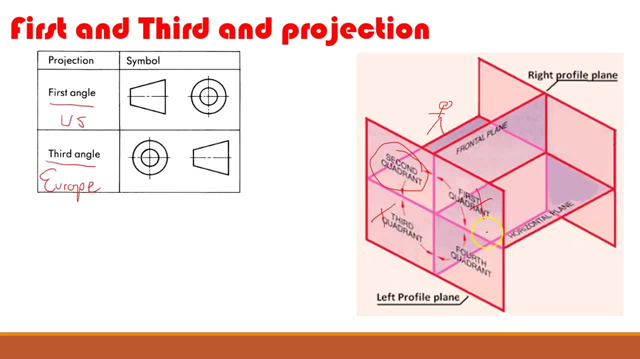 shift it. you don't twist it, you don't reorient it. you leave it in that same orientation, whether it's in the first or the third quadrant. so the difference between the first and the third quadrant observational point of view determines how you actually see this when you portray it in an 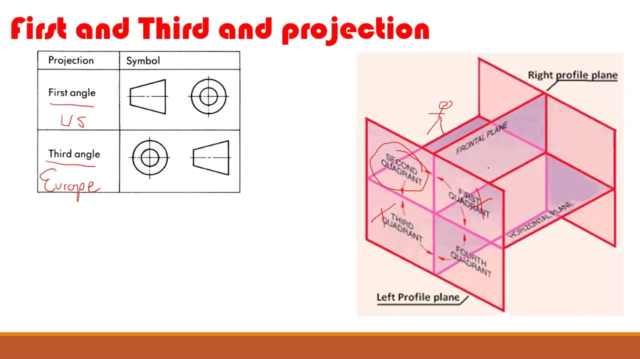 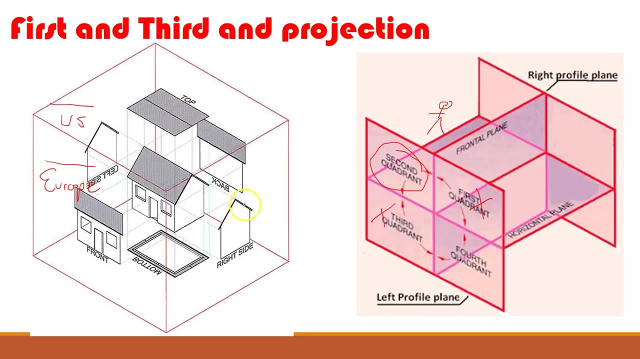 orthogonal point of view. so let's give this a little more clarity by looking at this drawing here. so what you have here is a house, and this house is pictured within a cube, an imaginary cube, and you can think of this cube, as you know, with orthogonal drawing. 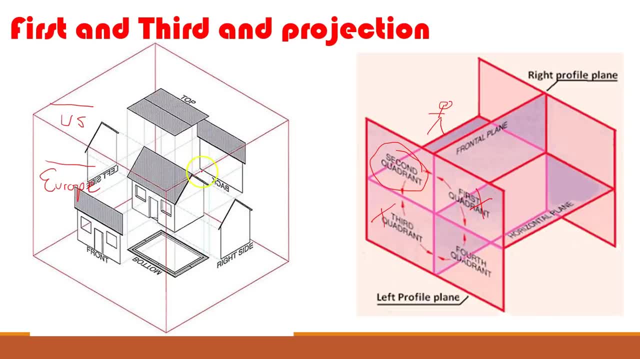 being projected onto each screen of the cube, on each face of the cube, so when you're in a first angle projection you know. in other words, it's sitting here in the first quadrant, you're in the second quadrant looking at this house, so that will put you over here. 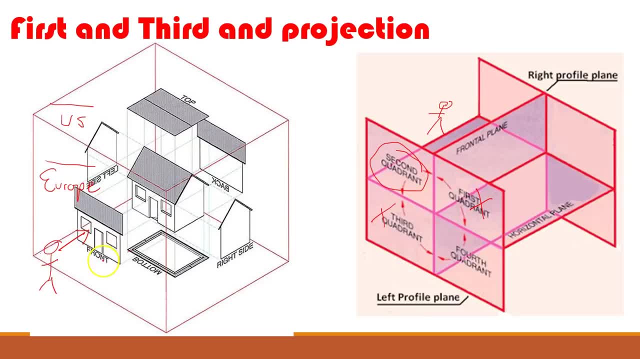 and you're viewing it this direction. this is why, in first angle projection you look at the front of the house and the side- right side- would fold out. you know, if we took this panel and folded it out, that would be part of your right angle or your your first angle projection you're looking at. 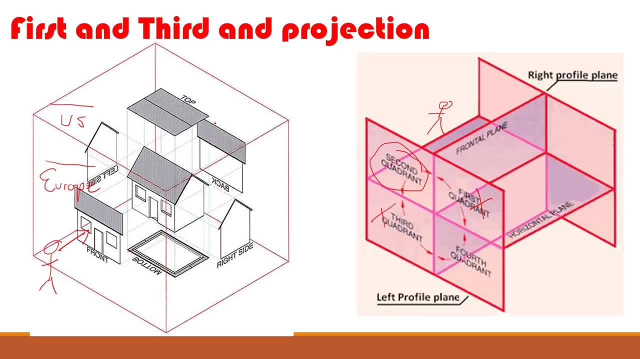 angle projection. your top would fold up above it, your bottom would fold down below it and your left side would fold out to the left. now, if you're looking at a third angle projection, you would have to picture yourself as sitting in the second quadrant, or you're still in the second quadrant. 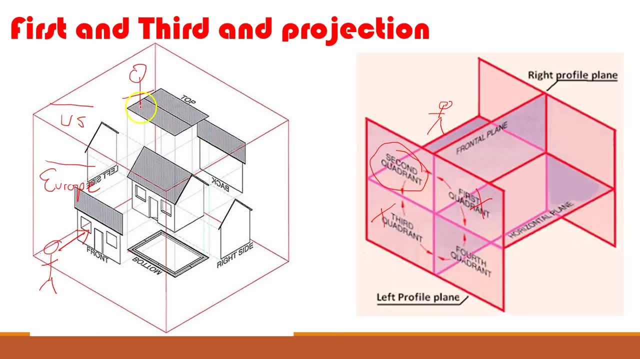 but the house is in the third quadrant and you're standing on top of the house and you're looking down, okay, so now the center of your drawing is going to be the top of the house. sorry about that. your center drawing is going to be the top of the house and below it is the front. 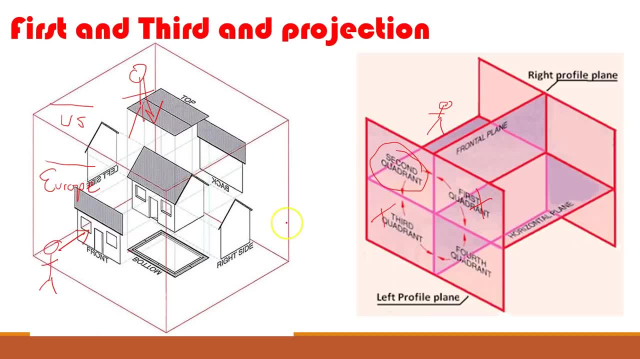 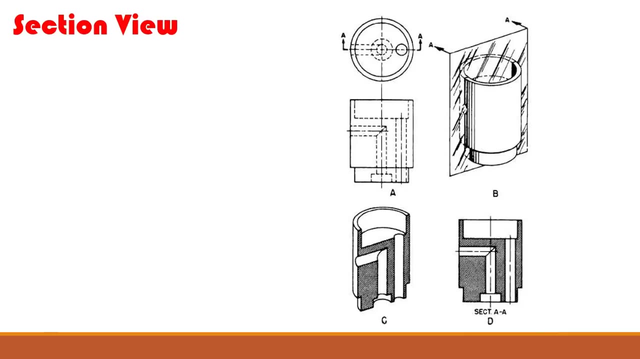 view as it folds out. the right side view folds out to your right, the back of the house folds above and the left side view goes out to your left, and that is the difference between a first and third angle projection. now another important view, particularly when you have a lot of internal: 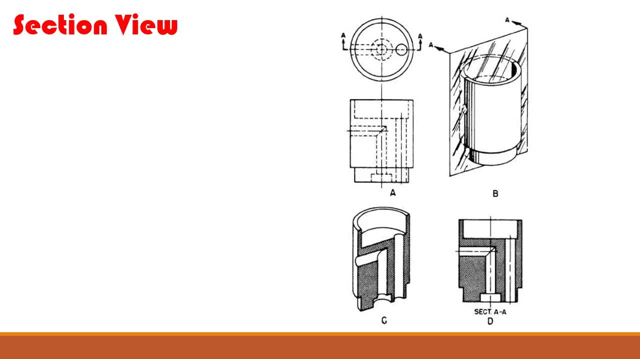 dimensions on our internal floor. you're going to want to make sure that you're looking at the angels. now for a table or side or whatever that you want. you're going to want to describe a row so we see the angle into the central nessa section of the inside, so as a full degree입wise. 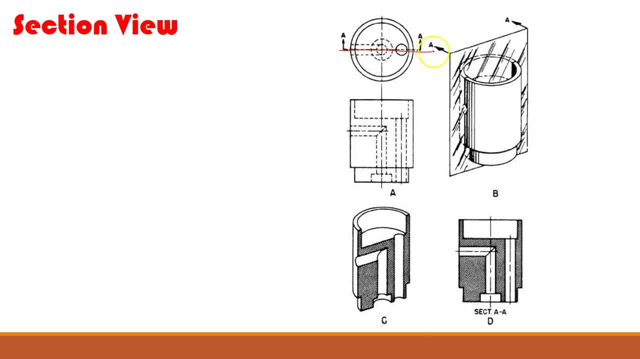 navigation. you're going to look at the outside, okay, and the side better. so the top of the house looks the same, with those little depressions located below between the hands. so that's where the half angle朝 and the outer angle of opening, the middle angle that you want to. 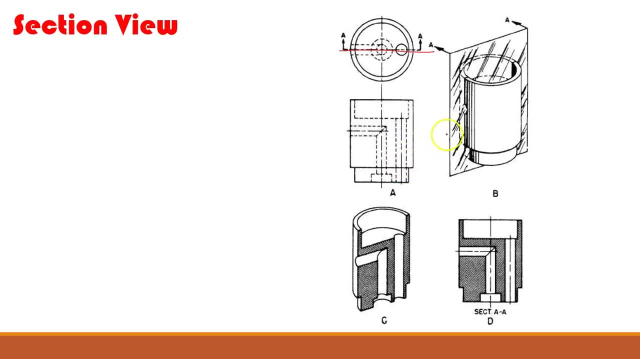 specify. so we already got all those things right, and now i'll leave that there after the video. so it's no longer this simple cylinder, it's a cylinder with several passages, and what we end up with is a section view that looks like this, you know. so it gives us the 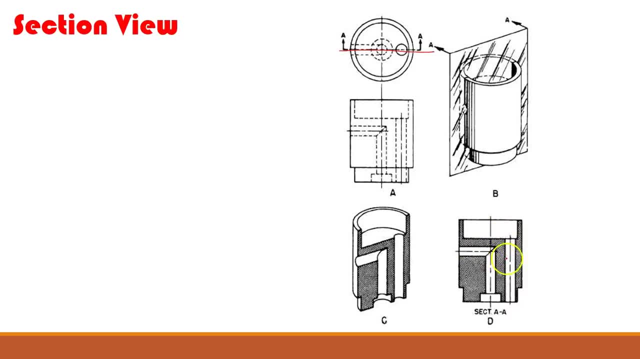 ability to see all the passages that might be going on or any type of internal workings in our component, we can actually dimension around some of these and actually understand what's going on inside of that, that part, and that's the importance of a section view. so it allows you. 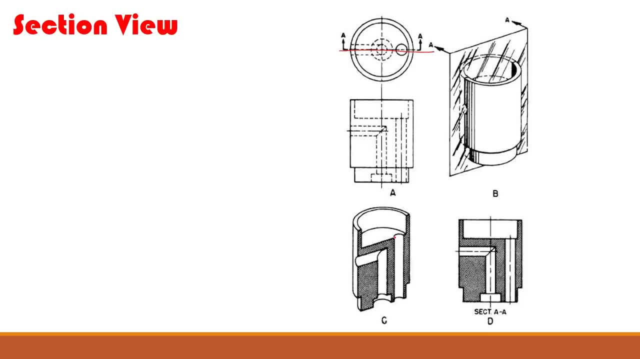 to see what's going on inside of the part you know it's. you know, while still maintaining some of your, your external sections. and the section view doesn't have to be a straight line, it can actually be a line that cuts across. you know, they could just easily, you know, show them the section. 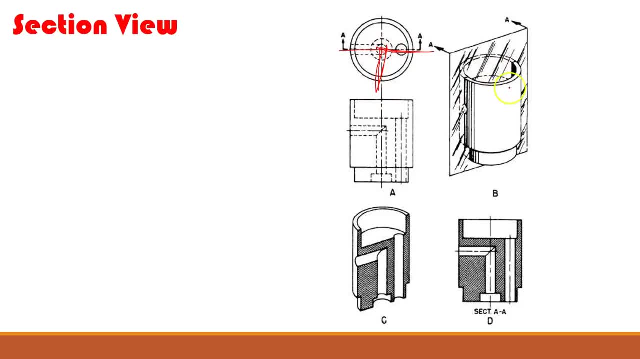 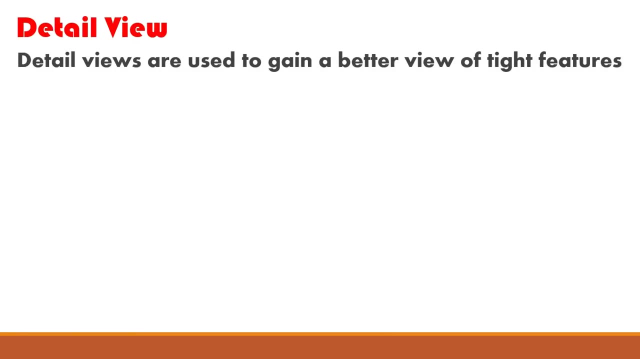 going along this in that particular path and have a 90 degree section cut out of the component so it shows normally hidden sections of a drawing. now the detailed view- it helps. it's the detail viewer are used to gain a better view of tight features. so if you have a 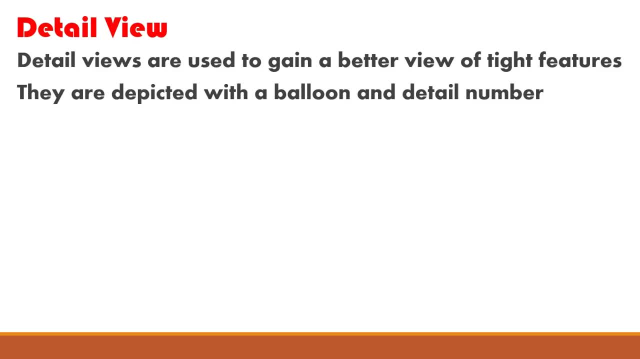 portion of a component that's just too tight to actually see what it is. you can actually use this detail view and it gets depicted in a balloon with a detailed number. so if you have this component here, you know whatever this particular is looks like some sort of a welder and you want to know. 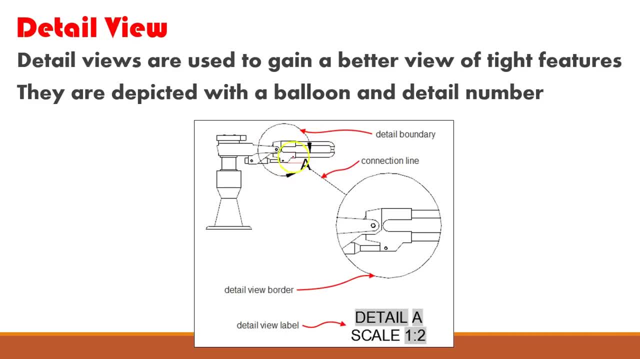 what's going on in this section a. so you have a detailed view, you open it up as detail day inside of a balloon or some sort of depiction, blows it up to a scale of one to two and now you can start to portray on exactly what is required in this component. you often see this detailed view. 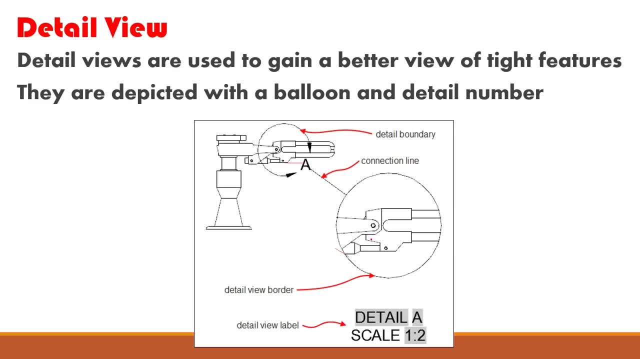 when looking at threading and looking at certain types of internal holes or any type of detail that might be too small and too below scale for the rest of your drawing. so you just use a detailed view, blow it up, put it in another section of your of your drawing, or on your on your blueprint. 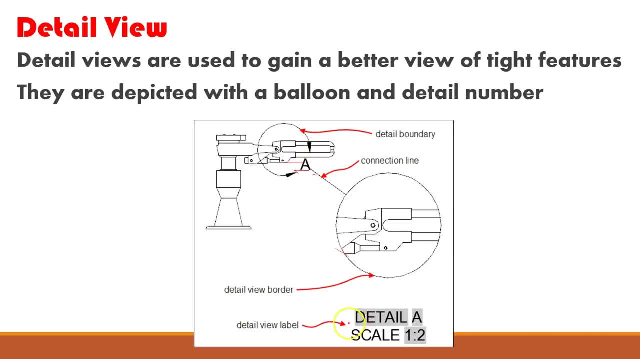 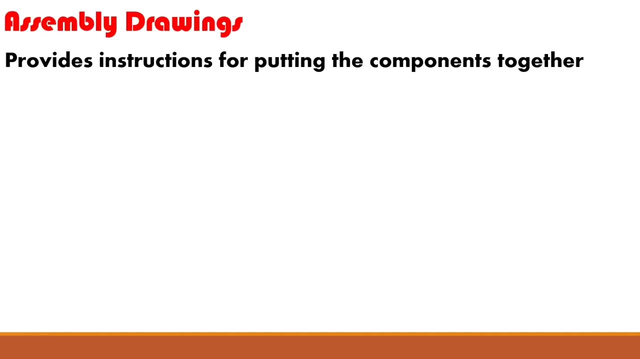 identify it, let it know that this section a is section a or detail a, and you're able to actually, you know, depict this compo part of your component on the same page. now you also got assembly drawings, you know. they provide instructions for how you would put that component together, you know, along with your title block, which is always a part of the 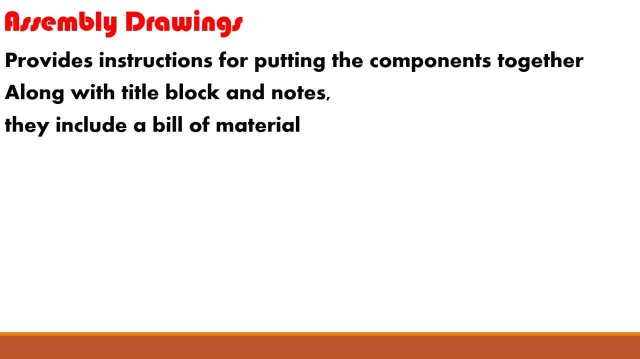 engineering drawing. you have what is known as a bill of materials, and all the bill of materials is like a grocery list of all the components in your in your, of all the different details inside of your component. so let's look at this particular drawing now, what we have here. 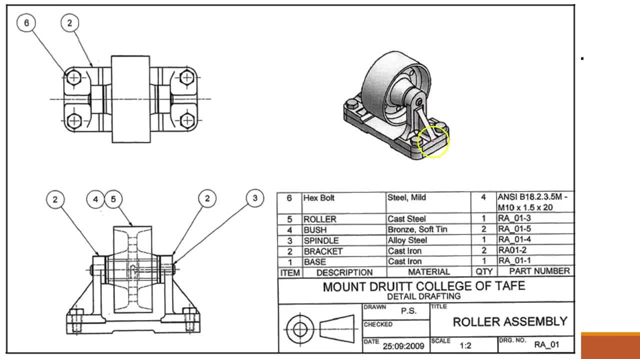 is some sort of roller assembly you can see. you've got your isometric view here so you can see what this looks like in all three dimensions. you know top front, bottom side, but on the left and right you have your drawing, which is no longer a single component, it's actually a full assembly of all. 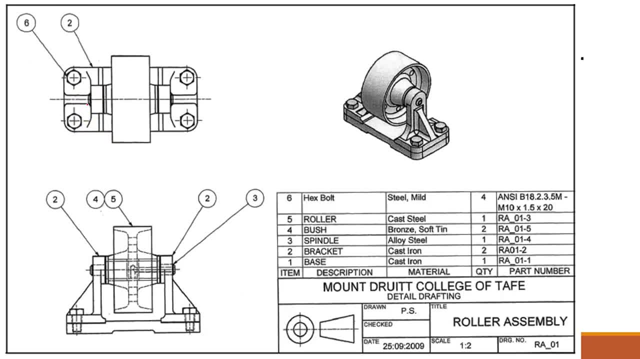 those components, so you can see that you've got both of them and you also have a lot of components: bolts, you've got a roller and you've got a base and you've got, you know, several things that are internal to them that you can't directly see, but they're all depicted with these little balloons. 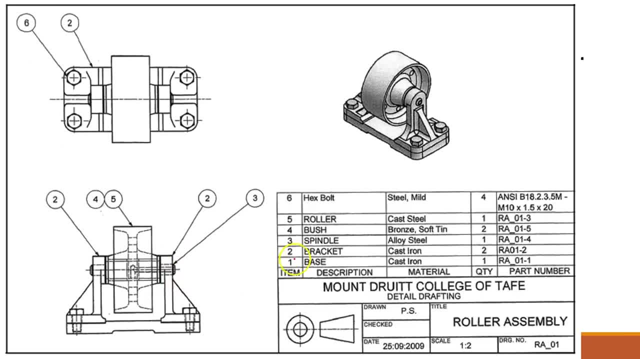 and numbered out, So you could say what part is what. Now, this bill of material is important because it lets you know not only what the component is, as they correlate to these balloons, but the quantity that you're going to require and what information you're going to need if you. 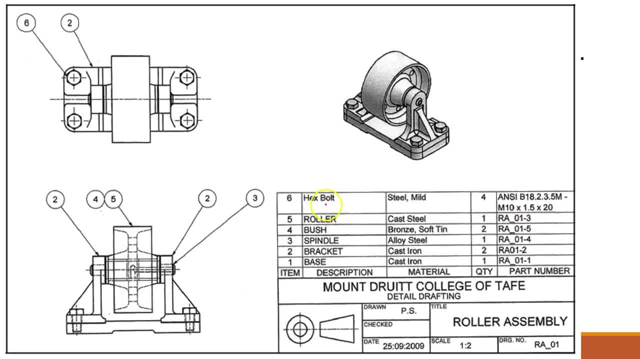 actually order the portion. So right here we've got detail. six are hex bolts. They're made out of mild steel. You've got four of them and this gives you your detail. So they're metric, 10 millimeter threads and you, you know, have enough information that if you needed to order some more, 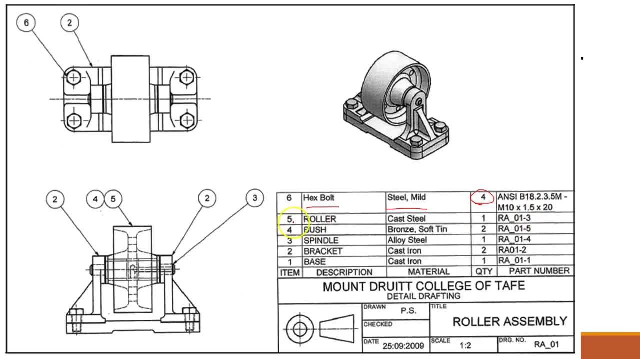 of these bolts you could very easily. Now you also have component five, which is the roller itself. You see this depicted here, pointing directly to the roller. This is made out of cast steel. you only have one, a quantity of one, and it is seen in part number ARA01-3.. So that lets you. 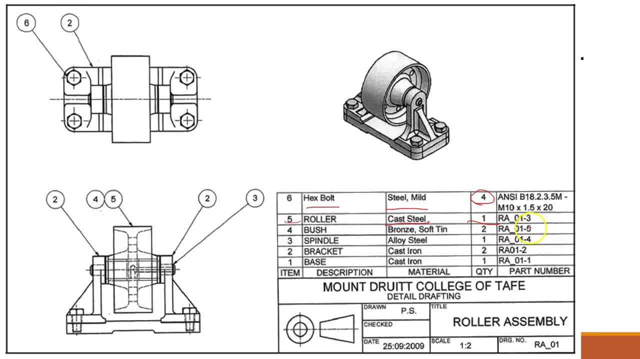 know, there's this, the details of this, with all the dimensions, you know, all of the tolerances, all the surface finishes is going to end up in this drawing. So this is the drawing you're going to need and you can see that all of these components have their own drawing with all of 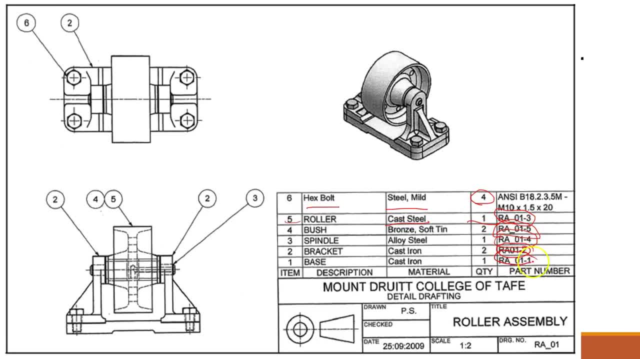 their separate dimensions and features. but just from this one drawing you're able to see exactly how this component is assembled And what all the parts are together and what they're made from. So this is a really important drawing because you could actually use this to actually order and buy more or get more. 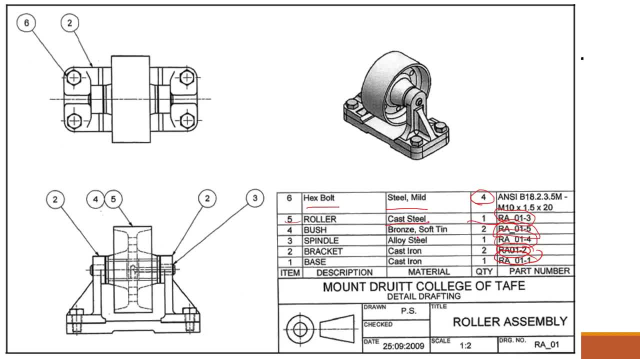 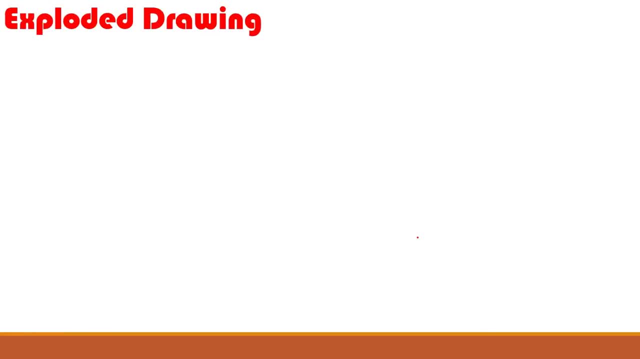 manufactured and still know how to assemble it together. So again, this communicates all the way from the design, in this case, all the way to the assembly process. Now, another good drawing is the exploded drawing. Now, this is a different type of assembly drawing, but it shows the 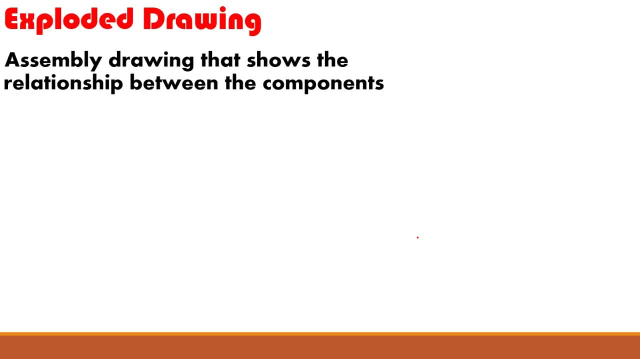 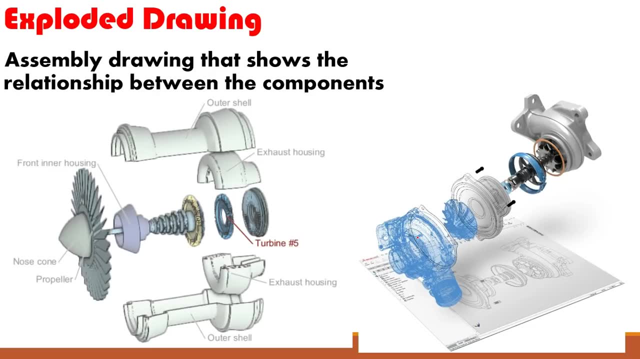 components all in relation to each other and how they're going to be assembled. So this is a kind of drawing. you see if you have a component or something you bought from, say, Ikea and you need to know how you're going to put it together. It actually shows all the components laid out and 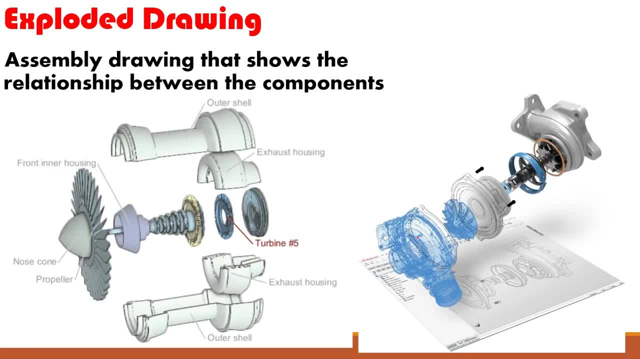 oriented, so their functional relationship is played out together. So you can look at this drawing and tell you, know that this turbo, how everything is going to assemble, So what part goes in first, second, third and fourth. So this is a kind of drawing. you see, if you have a component. 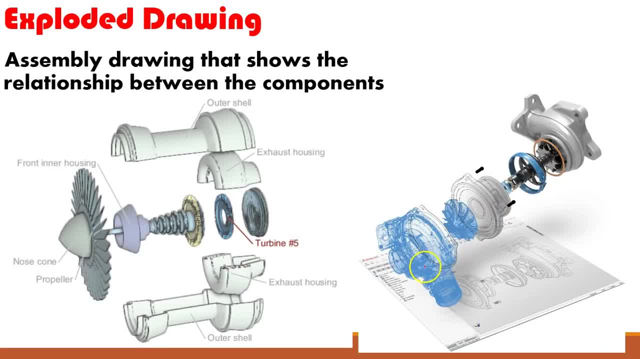 where the bolts are going to go in and then, finally, how the housing is going to be clipped on. On this portion you've got the outer shell, you know depicted, you know blown apart, you know from each other. You know, you got your outer shell and then you got all the internal. 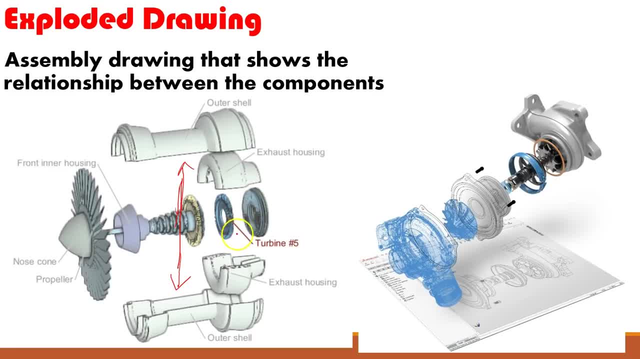 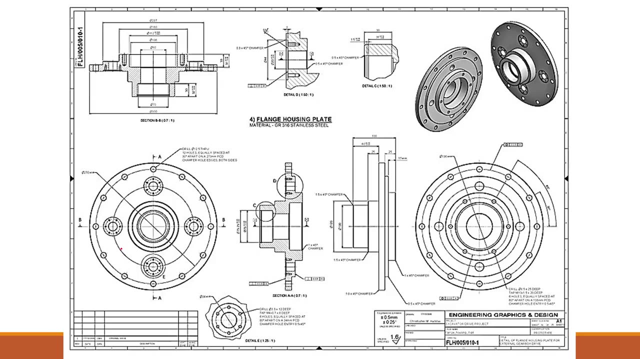 components: the exhaust housing, you know, you got this turbine number five, and you got the inner housing, the nose cone, the propeller, you know and how they all come together inside of that shell. So if you look at this particular drawing- I know it's a very busy drawing- we can see that pretty. 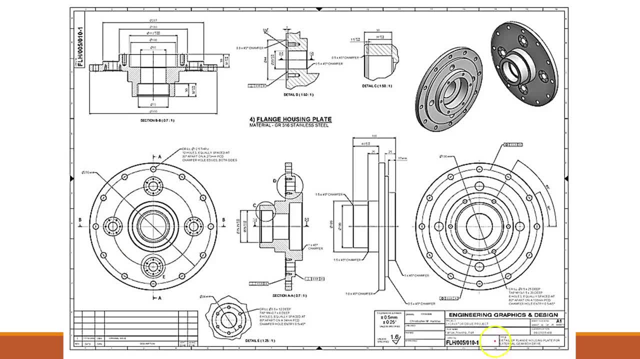 much everything we spoke about is here, So we've got the title block down here at the bottom. We know the company name is Engineering Graphics and Design. We got part numbers. We got the tolerances- universal tolerances and surface finishes depicted here. We got an isometric. 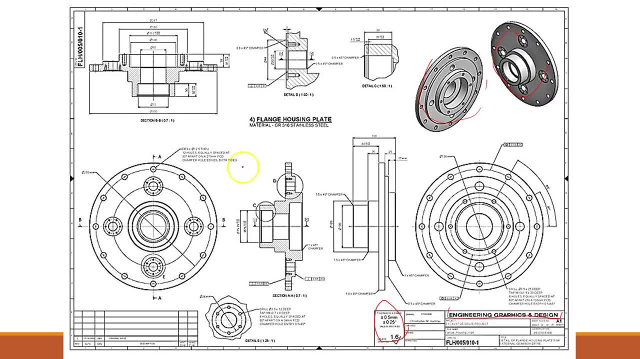 view. so we know exactly what it is we're looking at And you know it's a flange housing. We know it's made out of 316 stainless steel. We know it's a first order or first angle projection. We have a section view, section AA, that slices it right down the middle and we can see the internal. 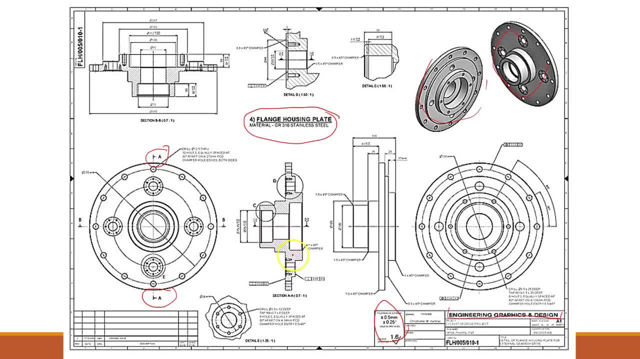 workings of this component. We see all the dimensions that we have here that we're going to be concerned with, the different types of threads, the difference of bolt holes, our screws. We also can see different types of detailed drawings. So we've got detail D which depicts this portion here. We got detail C which depicts this portion. 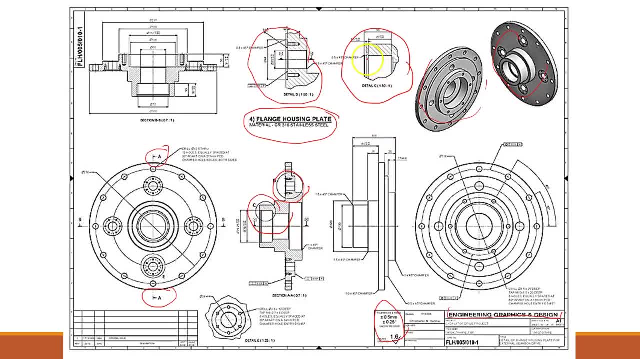 here. So now, because these are such small portions, we can see now what these snap rings look like. We can see much smaller and tighter tolerances. You can get more information on, you know, the different types of what might be an O-ring or a chamfer area inside of here that we couldn't have seen. 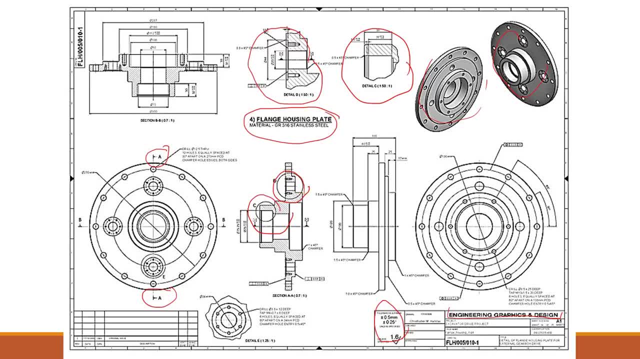 inside of this drawing. So what you can see is that this sort of detail here on the top right is going to be a little bit of a cutout on this one of a drawing. you know, this is a full functioning drawing of all the things that we spoke of, or most. 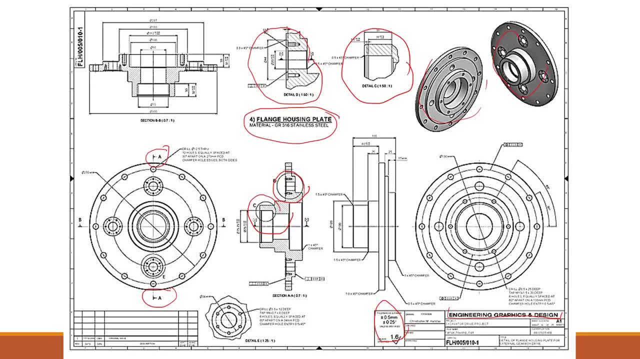 of the things we spoke of. that shows how this works in the real world now and you can see that you know. knowing all of these, you can reference back and start figuring out how to make this component, how to communicate it, and if you have a part that isn't made properly, you can actually go. 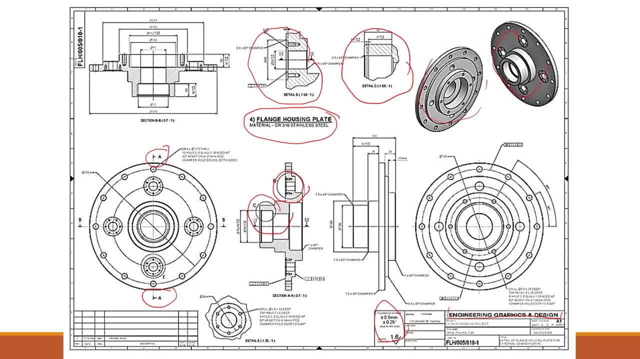 back to your supplier and address any issues. you can also see, just based off of the tolerances, exactly what you're going to do to manufacture this component, and well as how you're going to have to clamp it or restrain it when you do any type of inspection. 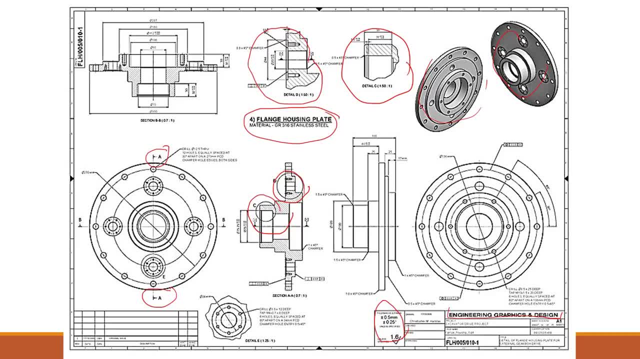 so that's some of the basics of engineering drawing and understanding an engineering drawing. if this was helpful, go ahead and subscribe to the channel, share it with anybody who might be struggling with engineering or any types of reading a blueprint. if you have any comments, you know, please let me know if there's any type of details that you would like to know more about in terms of.